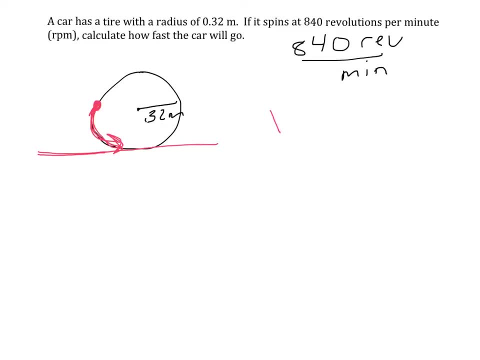 So in this situation it's velocity, and it really comes down to, like most velocity things, distance over time. So, at the end of this circle, what distance is being traveled over what period of time? And this right here, 840 revolutions per minute, is in fact the sort of velocity. 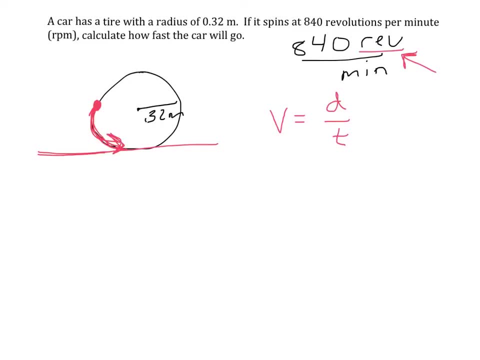 The revolutions represents the distance, and the minutes are the time, But that's not very useful to us. We usually want a unit like meters per second, So to figure that out we have to first find out, okay. well, what is the distance of one revolution? 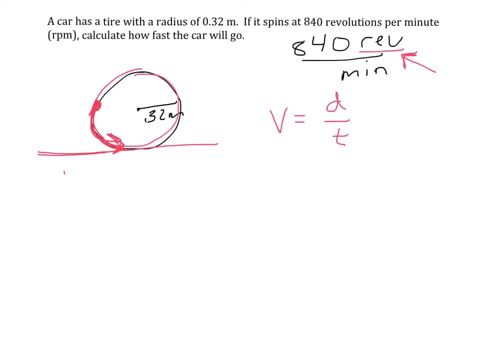 So a revolution is a complete time around the circle. So one revolution. we're going to use the formula for circumference, which is 2 pi r. So one revolution then, for the circle is going to be 2 pi times 0.32.. 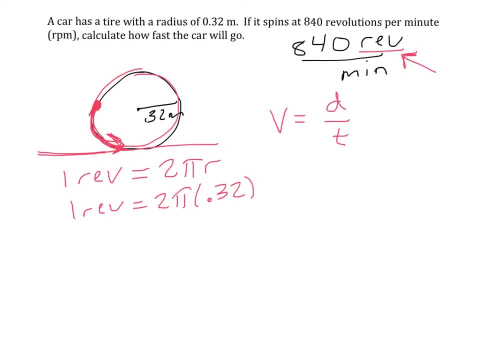 And so I'll plug that in, and so 2 pi times 0.32, I get that one revolution is 2.01 meters. Alright, so now I want to find out how fast this is going. I have 840 revolutions. 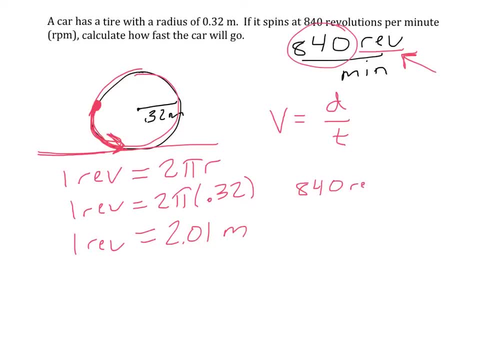 So 840 revolutions and one revolution. So 840 is 2.01 meters. so I find out what that distance is. So 840 times 2.01, and that is 1688.4 meters. So that, right, there is my distance. 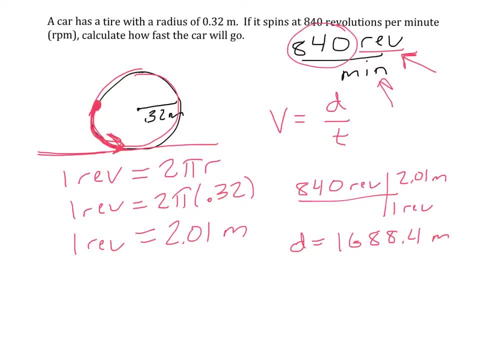 And now my time. it's in minutes, So if I want meters per minute I can divide by one and get that. But typically I'm going to want seconds. So I know that one minute and this I can just kind of do. the time is 60 seconds. 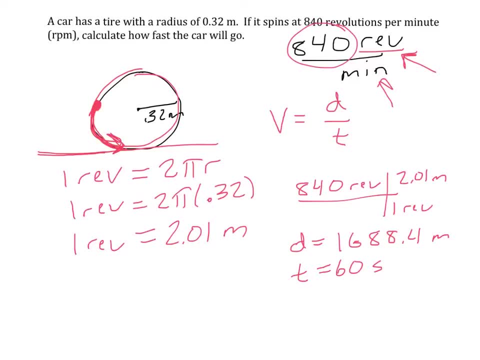 And if it was more than one minute then I could adjust accordingly. So now the speed of the car is going to be distance over time. So I'm going to say 1688.4 meters over 60 seconds, and that is going to give me my time in meters per second. 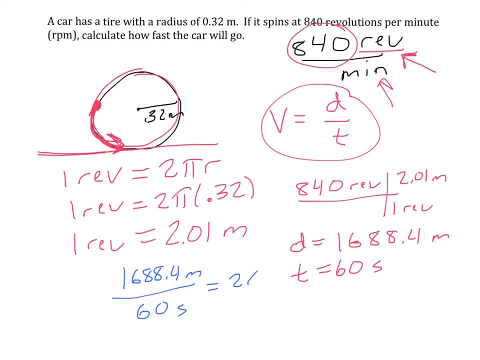 So when I do that I get 28.14 meters per second. I'll probably round this to 28.1 meters per second. Probably technically it should be 28 if I pay attention to sig figs, but I'll just call this. 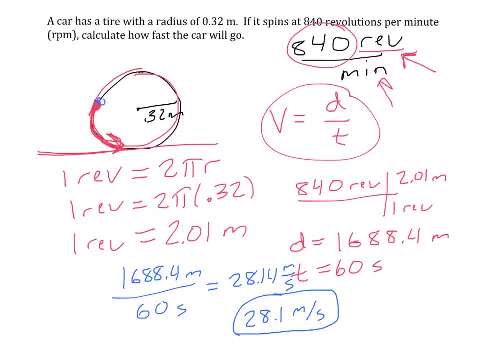 So that is the speed of the car And that's again, that's how fast. if you were on the edge of the tire, this is how fast it's going around in a circle. If the tire had a bigger radius and it was spinning at the same rate.